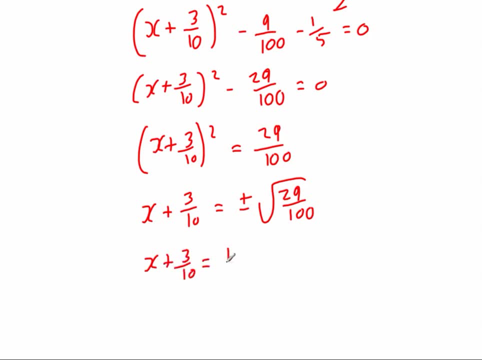 That's going to give us x plus 3 tenths equals plus or minus. the square root of 29 is just going to be square root of 29,, and it can't be simplified. But the square root of 100? Well, it's 10.. 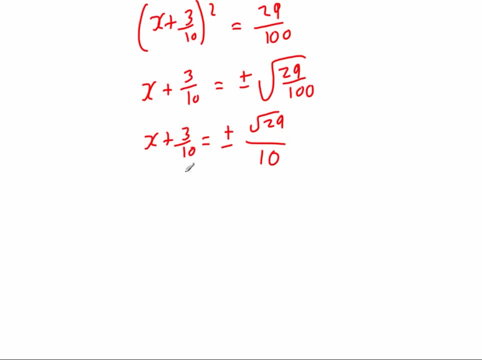 Next, we want to get rid of the plus three tenths, so we're going to take away three tenths. So it's going to be x equals. now, whenever I subtract or add this number here, what I do is I tend to put it in front of the plus or minus, so that's going to give us minus. 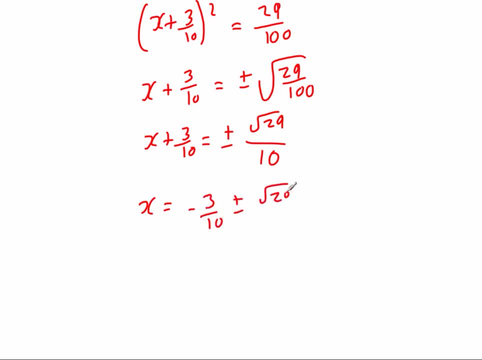 three tenths plus or minus the square root of 29 over 10.. Now we can just write it because it's got the same denominator. we can just write it as x equals we've got minus three over. sorry, because we've got the common denominator. 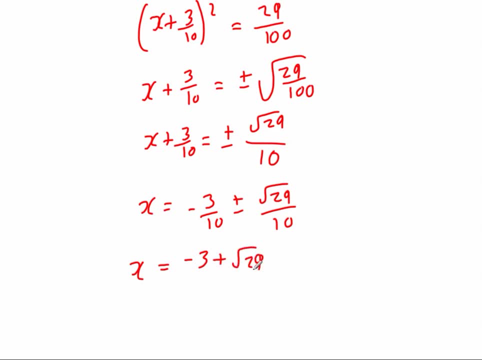 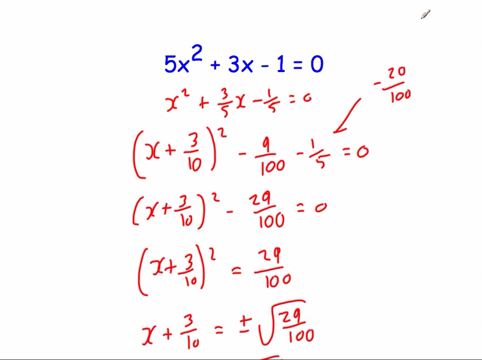 we can write: minus three plus root 29 over 10, and our other solution is: or x equals minus three minus root 29 over 10.. That's it, So that's how you can solve it, using completing the squares. So the main point to get you started is: because it was a five x squared you could divide. 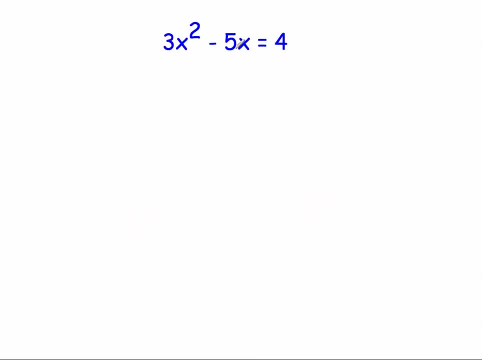 through by five, because it equals zero. The second one, then, is going to be very similar, so we're going to get three x squared minus five. x minus four equals zero. just bring it all over to one side. We're going to divide it through by three this time, so that's going to give us x squared. 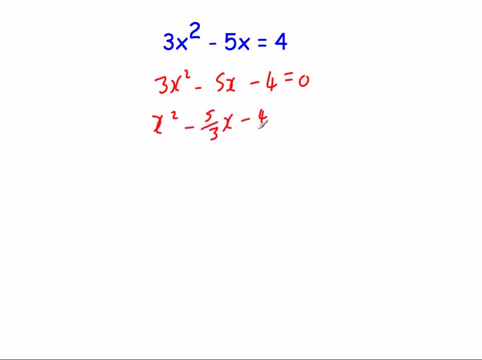 minus five thirds. x minus four thirds equals zero, And then we just use completing the squares, so we're going to get x minus five sixths squared Square this term, so it's going to be minus 25 over 36.. Okay. 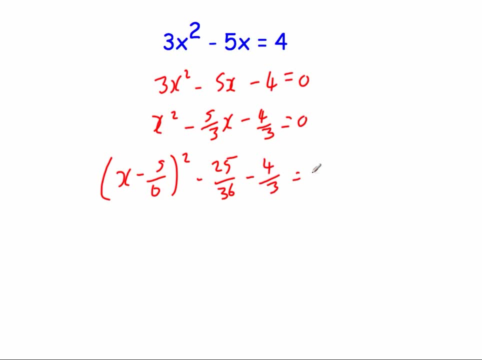 And then subtract four thirds equals zero. Four thirds we want as a common denominator. that's going to be 36, so it's going to be minus 48 over 36.. It's multiplying both of them by 12.. So that'll give us x minus five. sixths squared minus 25, take away over 48, that's going to.